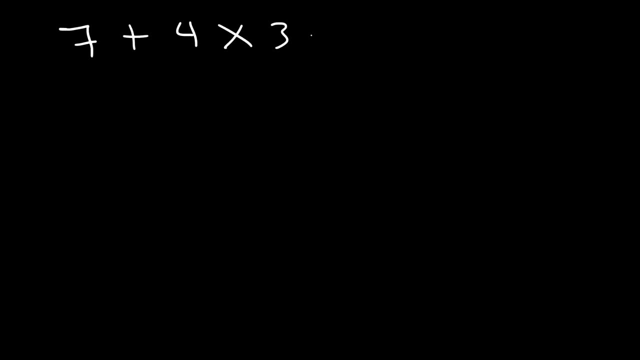 this: Should we add before we multiply, or should we multiply before we add? If we add first, 7 plus 4 is 11, and 11 times 3 is 33.. But if we multiply first, 4 times 3 is 12,. 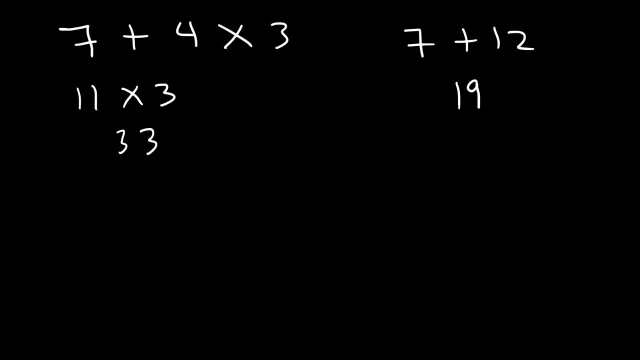 7 plus 12 is 19.. If you type this exact expression in a scientific calculator, it is going to give you this answer- 19, and not 33.. And the reason for that is because it's going to give you something called order of operations. There's a certain way in which you need to. 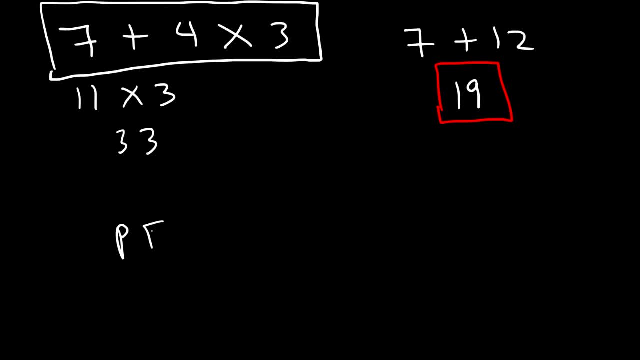 perform mathematical operations. Perhaps you've heard of the term PEMDAS, which is very helpful to know the order of operations Basically: P stands for parentheses, E is for exponents, M is for multiplication, D is for division, A is for addition, S is for. 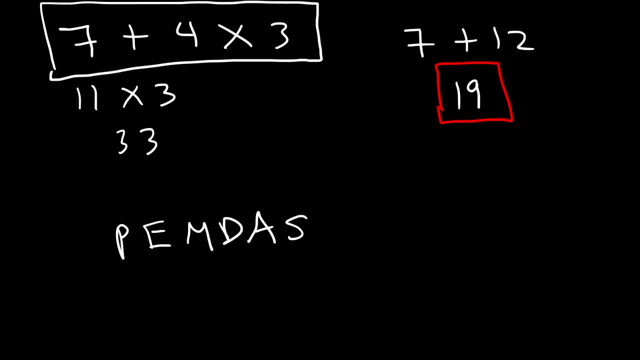 subtraction- So parentheses- has the highest order. Then come exponents, and then comes exponents. Multiplication and division are equal, and for addition and subtraction they're the same. So towards the left those operations have more priority. Comparing addition versus 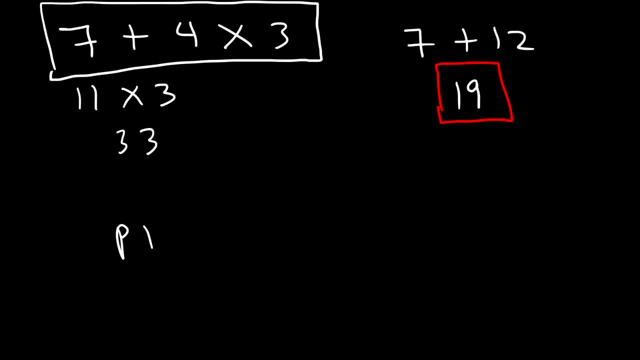 multiplication. Multiplication is on the left side, so we need to multiply first before we add, and that's why the answer is 19.. Here's another example: 36 minus 12 divided by 3.. So go ahead and take a minute and try this example Should. 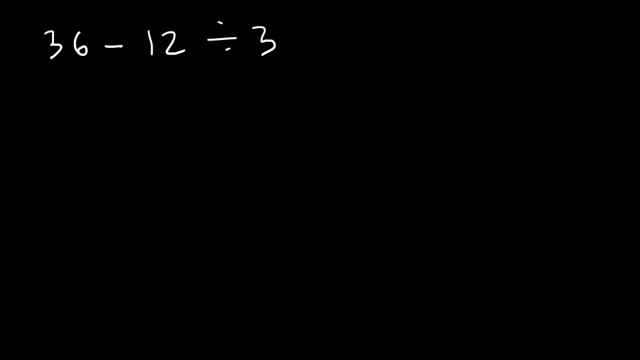 we subtract before we divide, or should we divide first and then subtract? Well, let's consider the expression PEMDAS. Notice that division has more priority than subtraction, since it's on the left side. So we need to divide first. 12 divided by 3 is 4, and 36 minus 4 is 32.. So that's the answer. 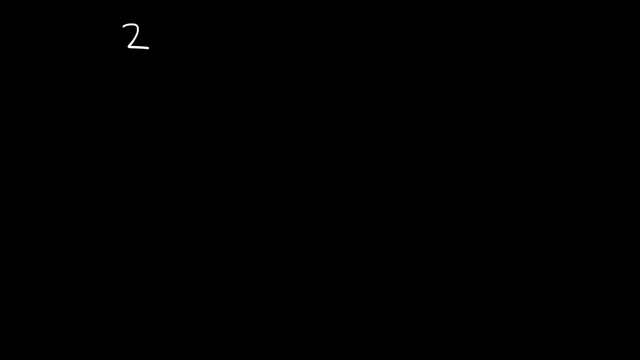 Now let's move on to our next example. What is 24 divided by 6 multiplied by 2?? Should we divide before we multiply or should we multiply first and then divide? Well, let's do it both ways. Let's divide first. 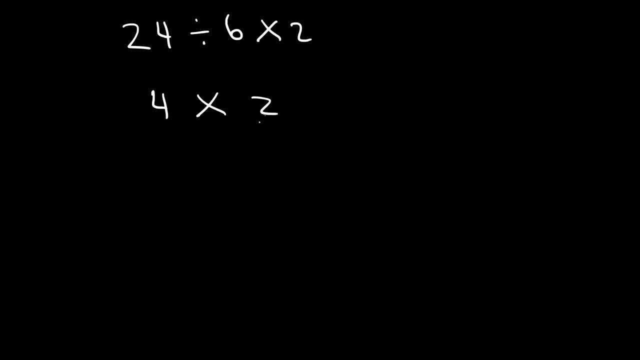 24 divided by 6 is 4.. 24 divided by 6 is 4.. 24 divided by 6 is 4.. And 4 times 2 is 8.. And 4 times 2 is 8.. Now let's do it the other way. Let's multiply 6 by 2.. That's going to be 12, and 24 divided. 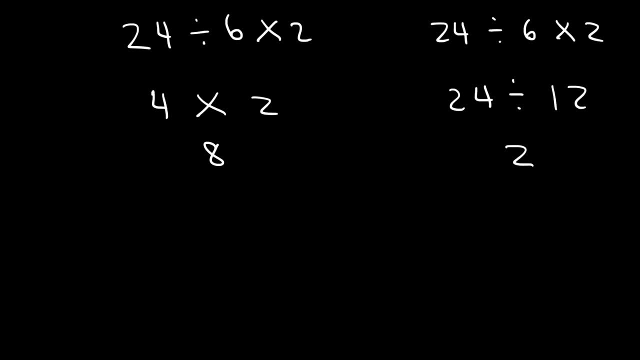 by 12 is 2.. So here we can see that we get different answers, so the order matters. If you type this expression in exactly the way you see it in your calculator, it will give you 8 as the answer. Multiplication and division: they have the same priority. so 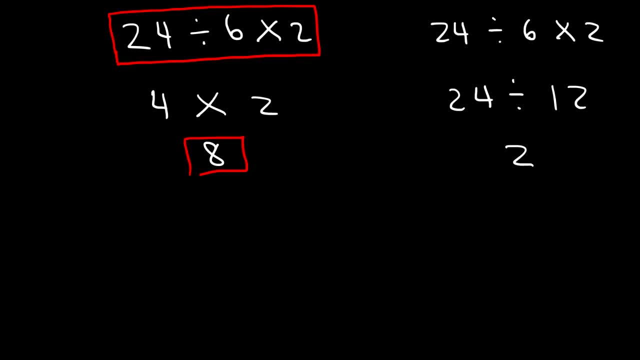 If you have a situation like this, the best thing to do is simply perform the operation from left to right, and it will give you the right answer. Another way you could see this expression is: 24 divided by 6 is a fraction, and then: 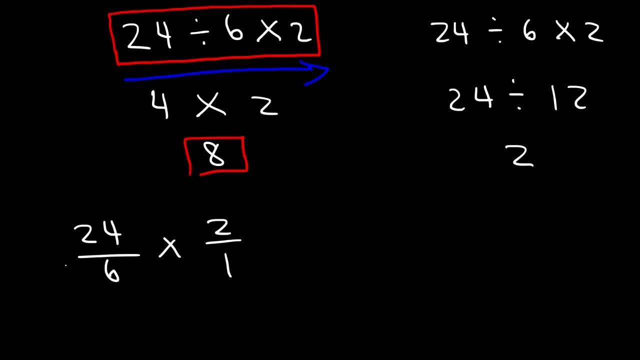 you're going to multiply by 2,, which is the same as 2 over 1.. So if you divide 24 by 6, you're going to get 4, and 4 times 2 is 8.. The other way to do this is to multiply 24 by 2,, which is 48,, and then divide it by 6.. 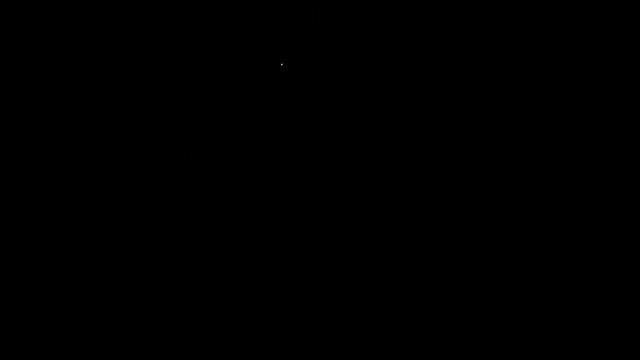 That will also give you 8.. Here's another one: 8 times 5, divided by 4.. So go ahead and try that. For this example, the best thing to do is simply to multiply from left to right. 8 times 5 is 40.. 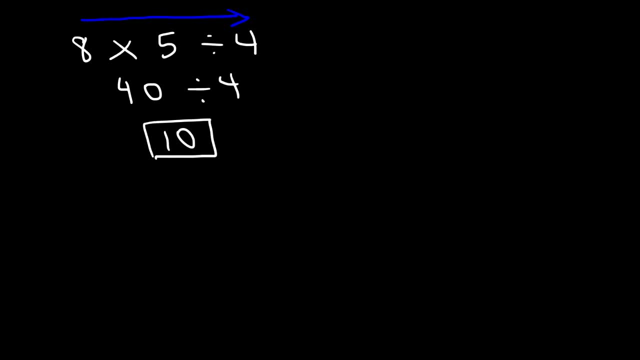 And 40 divided by 4 is 8.. And so that's going to be the answer. By the way, in this particular example, if you divide first, you're going to get the same answer: 5 divided by 4 is 1.25 as the decimal. 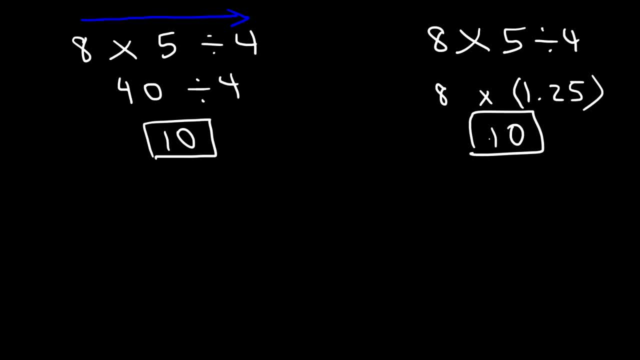 And if you multiply that by 8, this will also give you 10.. Try this example: What's 24 plus 12 divided by 10 minus 4?? Go ahead and see. Okay, Let's simplify that expression: 24 plus 12 is 36.. 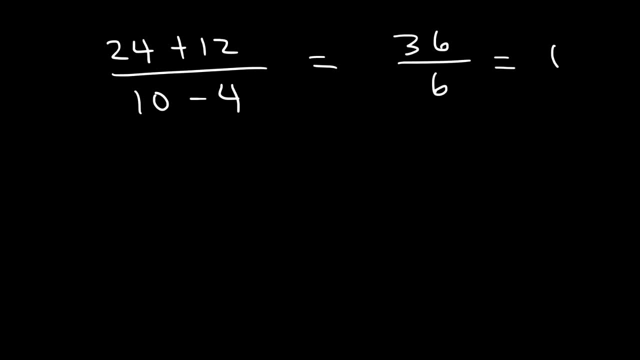 10 minus 4 is 6.. 36 divided by 6 is 6.. And that's all you got to do for that one. What is 4 multiplied by the sum of 3 plus 5 minus the product of 7 and 2?? 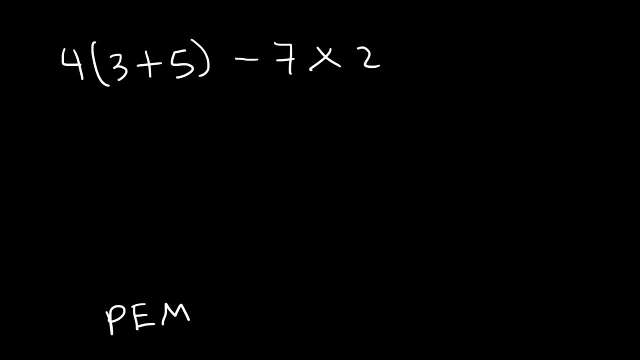 Now going back to the PEMDAS expression, Parentheses Has The highest priority compared to multiplication and addition And subtraction. So we got to work the operation that's inside the parentheses. first, 3 plus 5 is 8. And now we need to multiply. 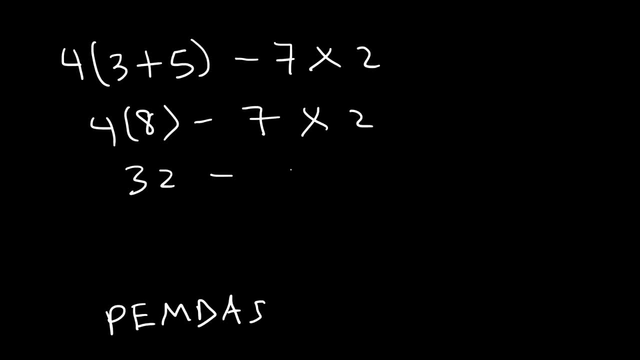 4 times 8 is 32.. And 7 times 2 is 14.. And now we can subtract 32 minus 14.. That's going to be equal to 18.. And so That's the answer for This example. 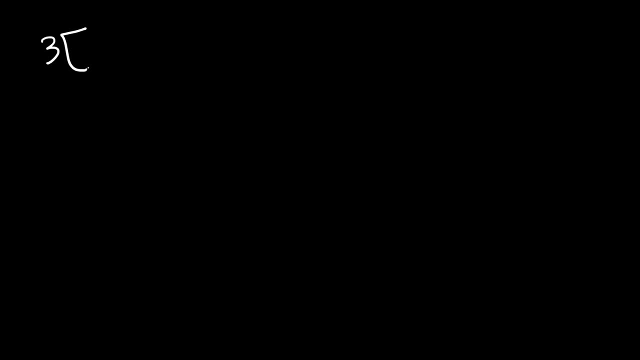 Here's a harder example that you could try: What is 3 multiplied by 4 minus 2 times 3 to the 3rd power minus 2 to the 4th power plus 8 times 2?? So the first thing we need to do is work on the inside of the parentheses. 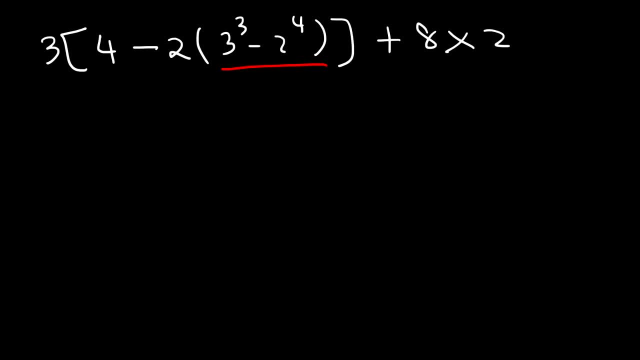 So we got to start Deep within the brackets. Now we have some exponents. So what is 3 to the 3rd power? When you're dealing with exponents, you need to think of it as repeated multiplication. Basically, this means that we're multiplying 3- 3's together. 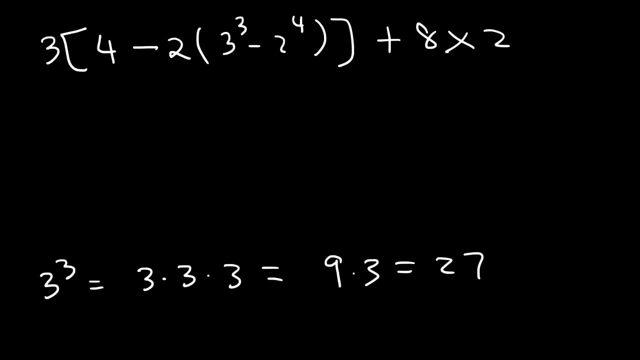 3 times 3 is 9. And 9 times 3 is 27.. So 3 to the 3rd is 27.. Now what about 2 to the 4th? So this expression means that We're multiplying 4- 2's. 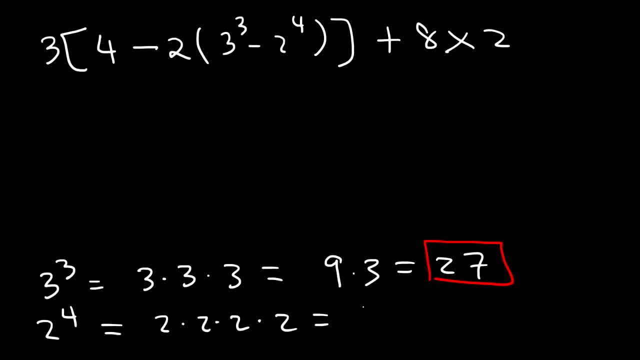 Together, 2 times 2 is 4. And 4 times 2 is 8.. 8 times 2 is 16.. So 2 to the 4th is simply 16.. So Right now, this is the expression that we currently have. 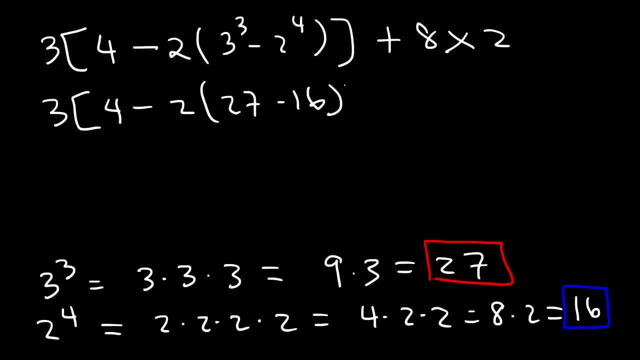 So We have 27 minus 16 on the inside And 8 times 2. we could just go ahead and make that 16.. Okay, Excellent. Now what is twenty-seven minus sixteen? Twenty-seven minus sixteen is eleven. Next, we have eleven times two, which is twenty-two. 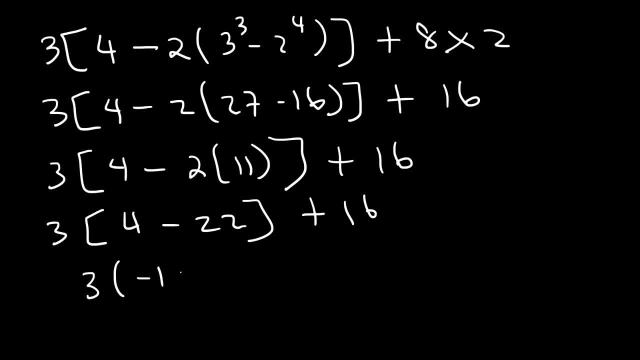 And then we have four minus twenty-two, which is negative eighteen, And three times negative eighteen, that's negative fifty-four. Another way in which you could do that is think of eighteen as being ten plus eight. Three times ten is thirty and three times eight is twenty-four. 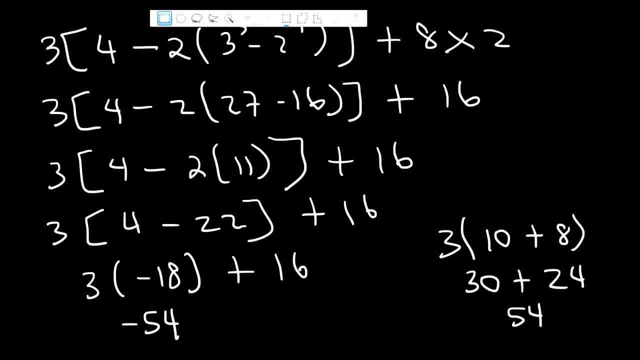 Thirty plus twenty-four is fifty-four. Now you can also do it this way: Eight times three is twenty-four. carry over the two: three times one is three plus two, that's five. That works as well. So now we have negative fifty-four plus sixteen. 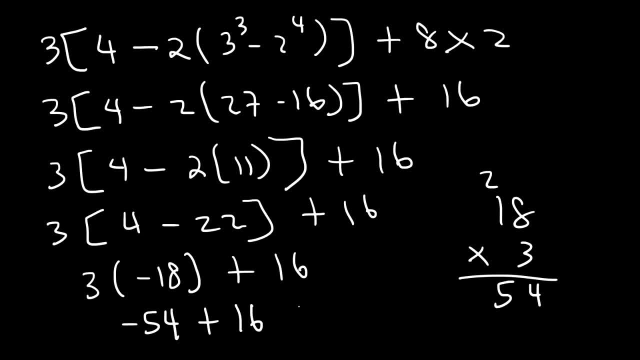 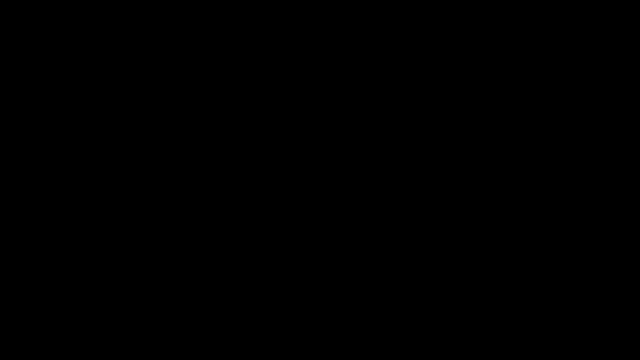 And if we use the calculator for that, this should give you negative thirty-eight. So that's the answer for this expression. Now let's say, if we have an expression that contains the variables four, x plus two, y minus three, z, Z is equal to two, y is equal to three and z is equal to negative four. 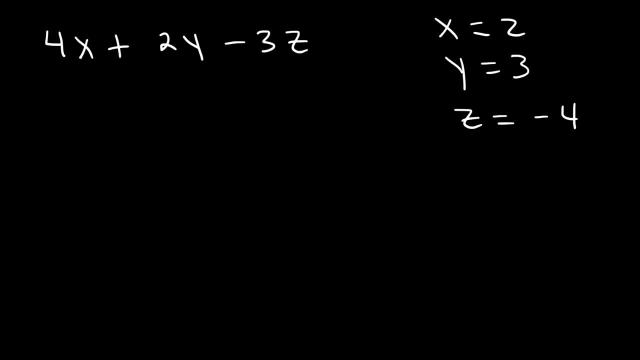 Go ahead and evaluate this expression. So what we need to do is substitute. We need to replace x with its value. X is equal to two, So let's replace it with two, And then let's replace y with three, And then we're going to substitute z with negative four. 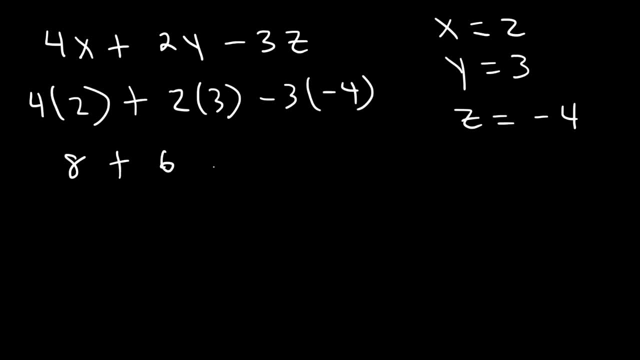 Four times two is eight. Two times three is six. Negative. three times negative four is positive. twelve. Eight plus six is fourteen. Fourteen plus twelve is twenty-six. And that's how you can evaluate an algebraic expression. Here's another example.